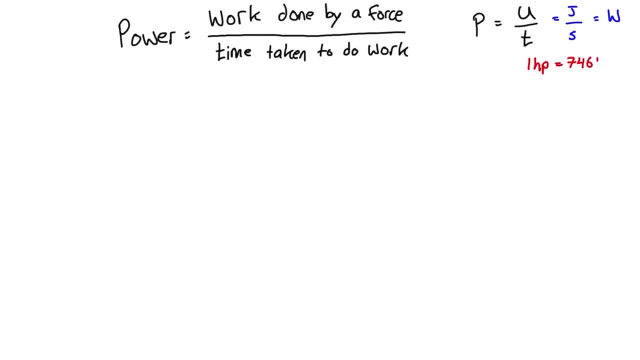 One horsepower is just equal to 746 watts. So let's just run over a simple example here. Let's say we have some kind of electric motor that's lifting a mass up three meters with a constant velocity in a time of six seconds. So let's say its mass is: 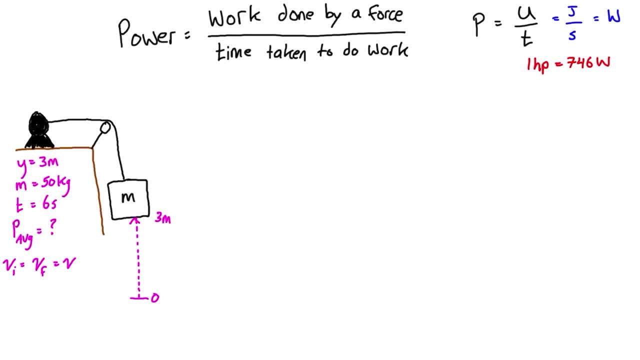 50 kilograms And let's find what the average power is required to make this happen. So we'll start with the conservation of mechanical energy equation, which is T1 plus V1 plus sum of work from one to two is equal to T2 plus V2.. So the capital T's are mechanical energy. 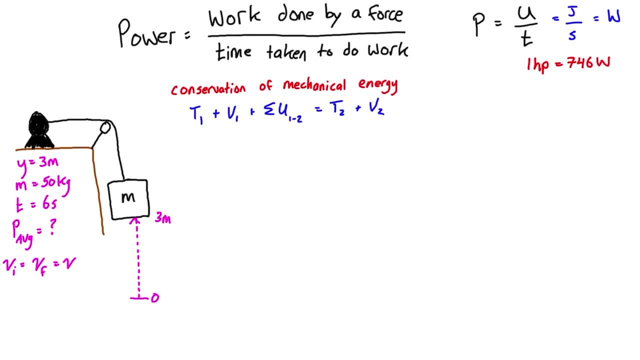 The capital V's are potential energy And U is the sum of work basically done between state one and state two. So we can go and expand this. Let's write: one half M V1 squared plus MGH, plus the work, is equal to one half M V2 squared. 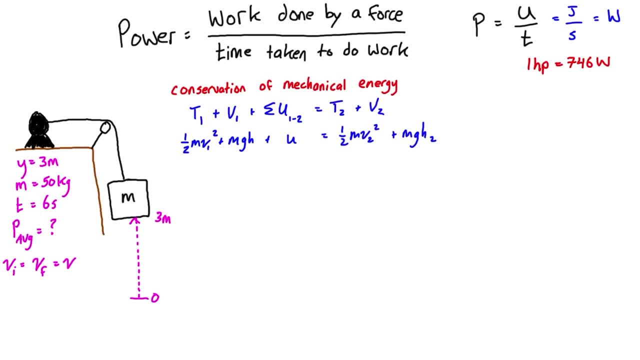 plus MGH2.. So right away we can cancel out the term for potential energy one, because H1 is equal to zero. This is maybe. let's write it like this: Let's say this is equal to H1,, whereas this is equal to H2.. 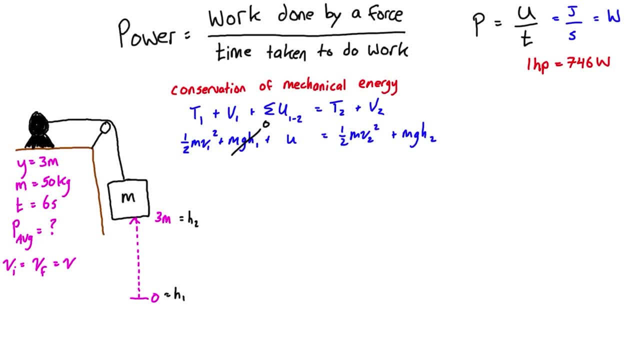 So H1 is a zero. it makes that whole term go to zero. And because velocity one is equal to velocity two, which is equal just to some generic constant velocity, we can subtract one half M V squared from both sides, And those terms are actually going to drop out as well because of that. So this just 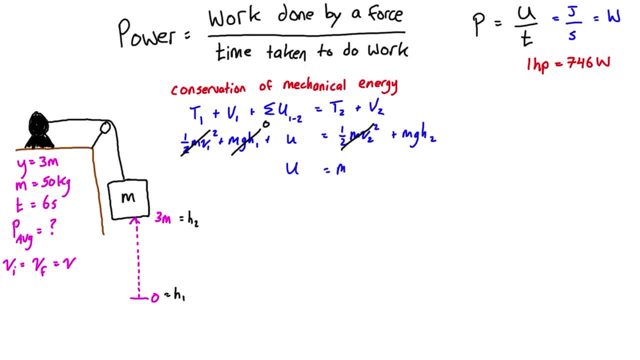 leaves us simply with the work done from state one to two is equal to MGH2.. And if we plug in the values that we have for that, it's 50 kilograms times 9.81.. Meters per second squared times H2, which is three meters. And that all simplifies to the work being 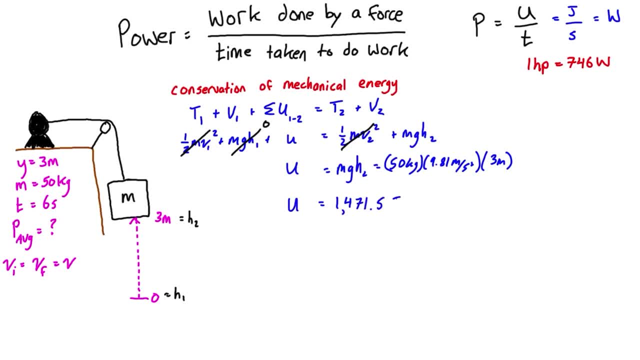 equal to 1471.5 Joules. So now, if we plug this into our power equation, where average power is equal to work done over the time taken to do the work, then we can just write it as P average is equal to u over T and we just plug in.